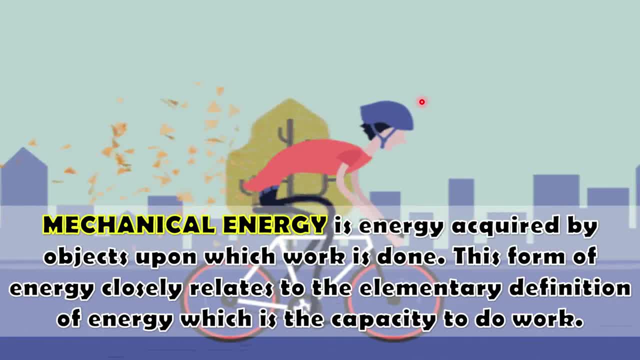 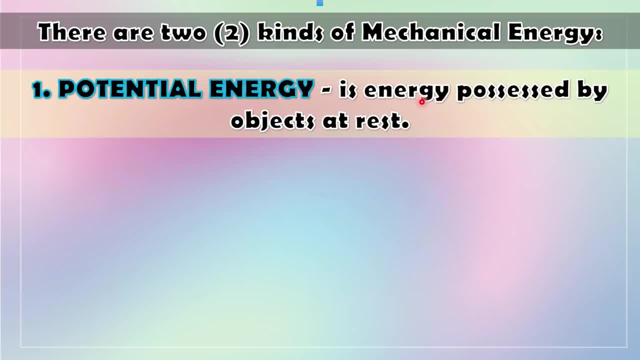 This form of energy closely relates to the elementary definition of energy, which is the capacity to do work. There are two kinds of mechanical energy. The first one is the potential energy. It is the energy possessed by objects. at rest, It has two kinds. 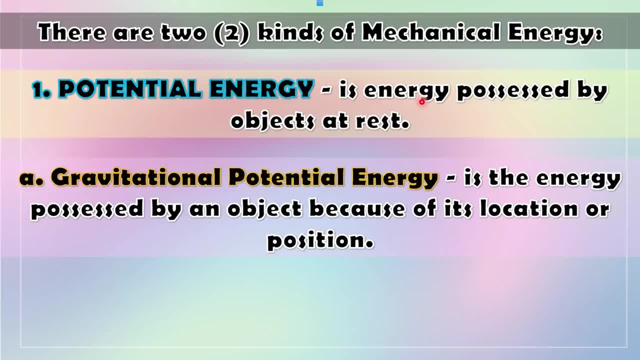 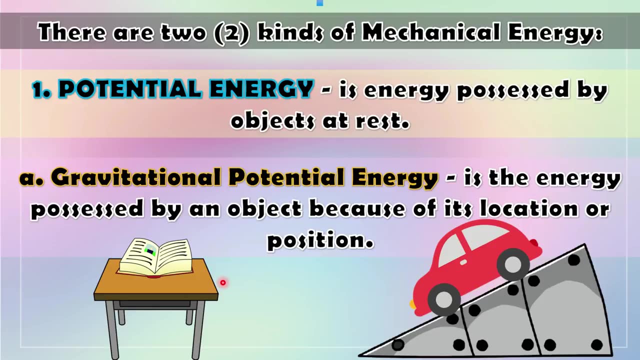 The first one is the gravitational potential energy. It is the energy possessed by an object because of its position or location, For example, a book on top of the table or a car parked on a ramp. These are examples of potential energy, because they possess energy due to their position or location. 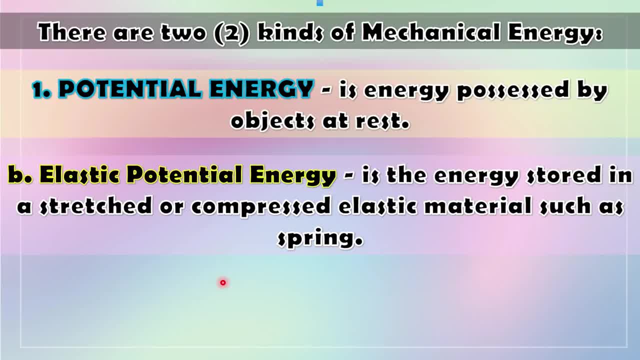 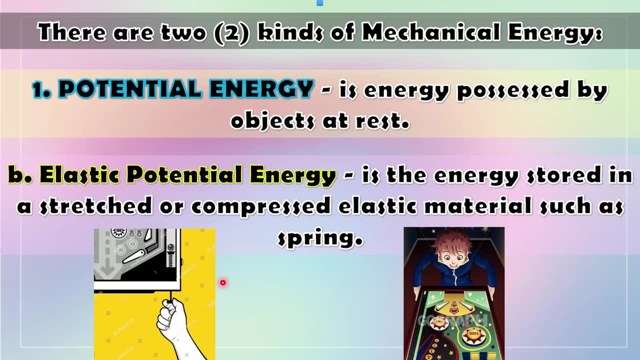 Second type of potential energy is elastic potential energy. It is the energy stored in a stretched or compressed elastic material such as spring. For example, the spring on the handle of the pinball machine has more energy when compressed than when in a relaxed position. 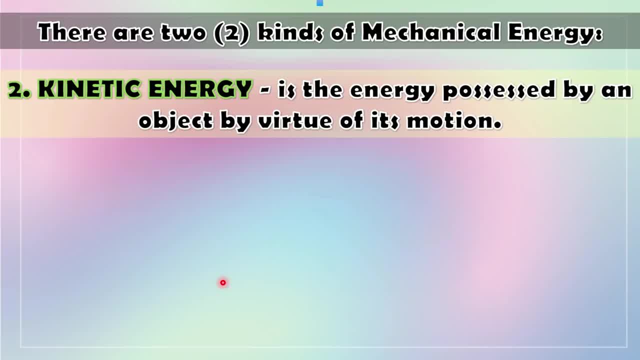 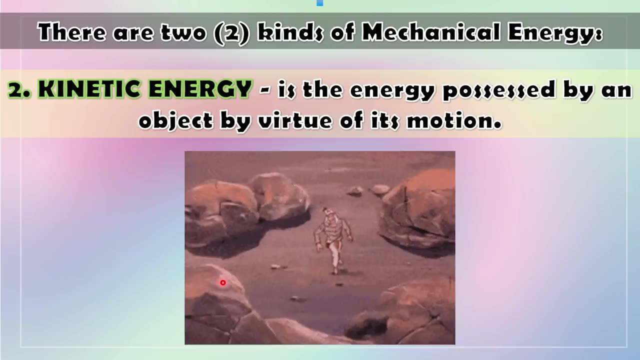 Second type of mechanical energy is what we call kinetic energy. It is the energy possessed by an object by virtue of its motion, Examples of which are a bullet in motion stream of flowing water, rock falling off a cliff and a rock falling off a cliff. 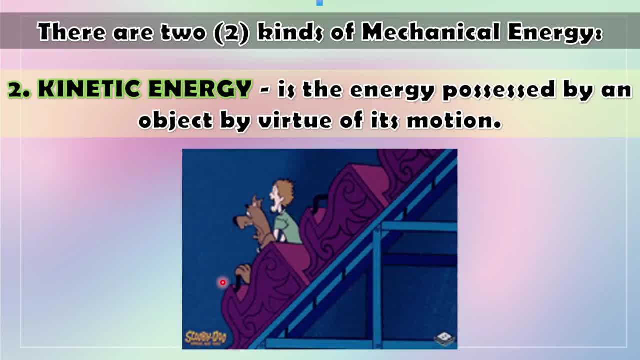 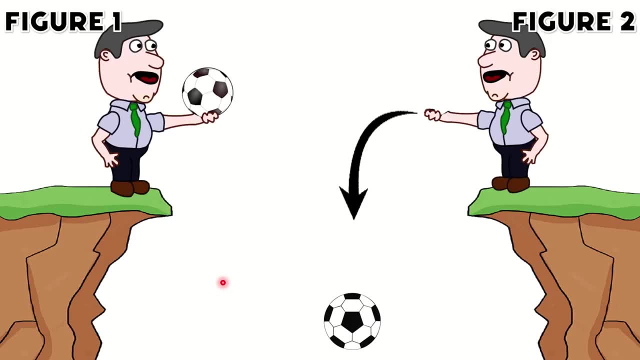 And a roller coaster. As you can see, they have energy due to their motion. Let us have this illustration for you to understand more. Shown in your screen right now is an illustration showing potential energy and kinetic energy. Again, class potential energy is the stored energy by an object due to its position. 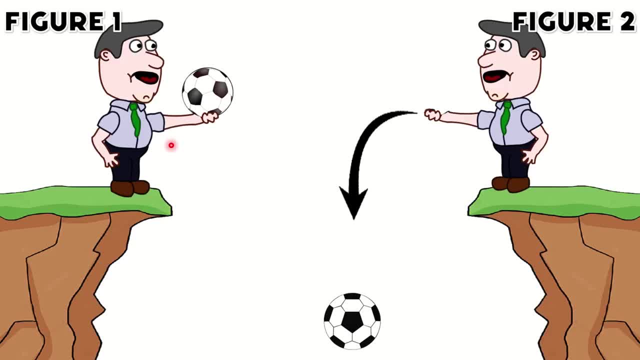 In figure 1, it shows a man holding a soccer ball. It is an example of potential energy. The ball stored potential energy due to its position or height from the ground. On the other hand, figure 2 shows kinetic energy. Again, it is the energy due to change in position. 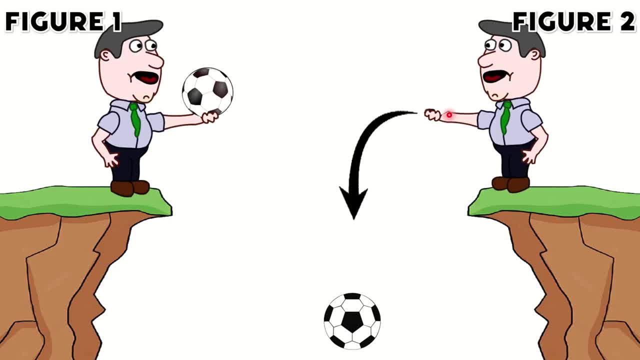 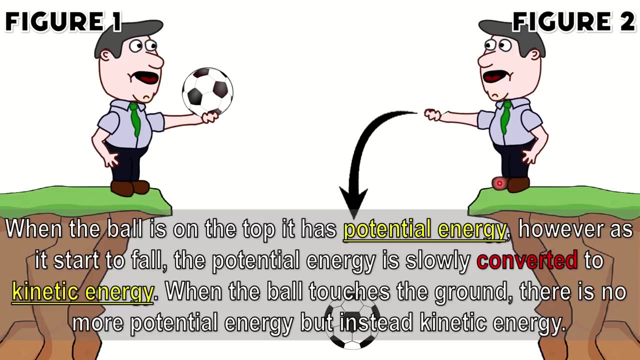 It is also termed as energy of movement or in motion. The energy associated to the change in position of the ball as it dropped is called kinetic energy. as shown in this figure, When the ball is on the top, it has potential energy. However, as it starts to fall, 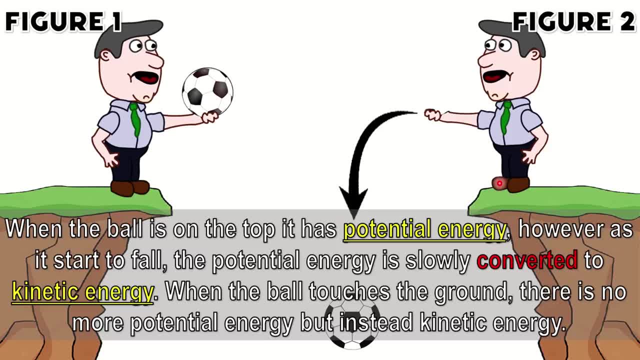 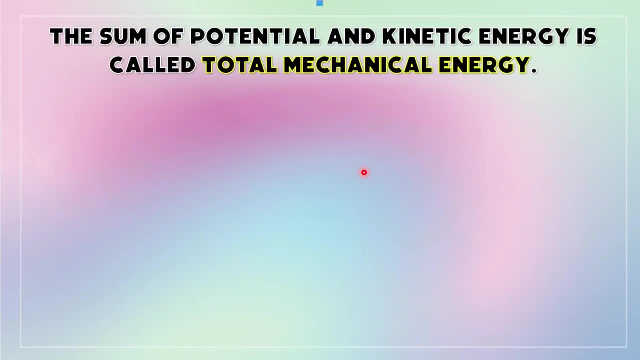 the potential energy is slowly converted to kinetic energy. When the ball touches the ground, there is no more potential energy but instead kinetic energy. Taking out of that class, potential and kinetic energy are forms of mechanical energy, And the sum of potential and kinetic energy is called total mechanical energy. 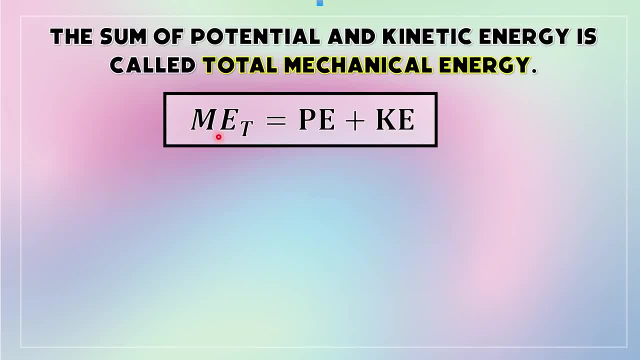 Mathematically it is expressed as: ME sub T is equal to PE plus KE, where ME sub T is the total mechanical energy and PE is the potential energy and KE is the kinetic energy. There are some instances that total mechanical energy is expressed as PE. 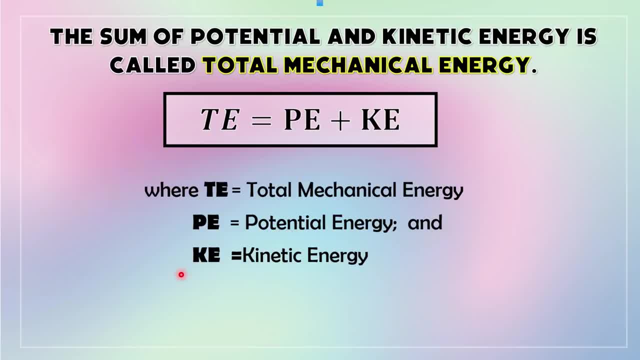 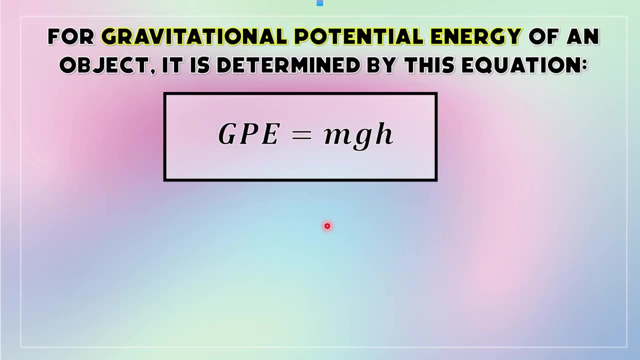 And again, it is the sum of the potential energy and kinetic energy. The unit that we are going to use for this is Joules. It is represented as letter J For gravitational potential energy. it is determined by this equation: GPE is equal to. 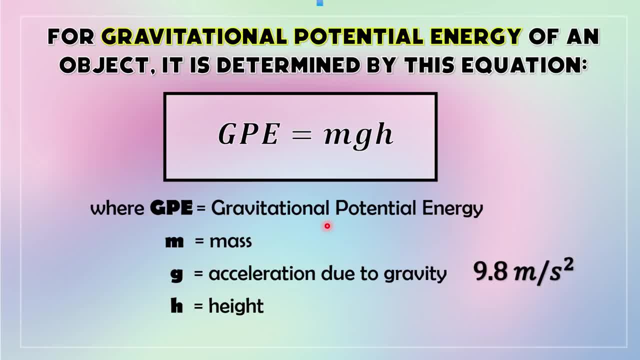 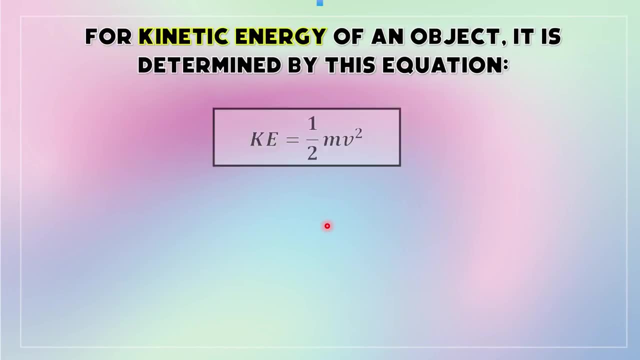 MGH, where M is the mass of the object, G is the acceleration due to gravity, which is 9.8 meter per second squared, and H is the height or the elevation of the object. For kinetic energy of an object in motion, it is determined by this equation. 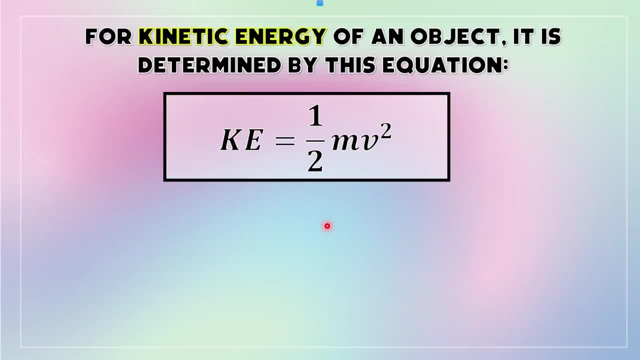 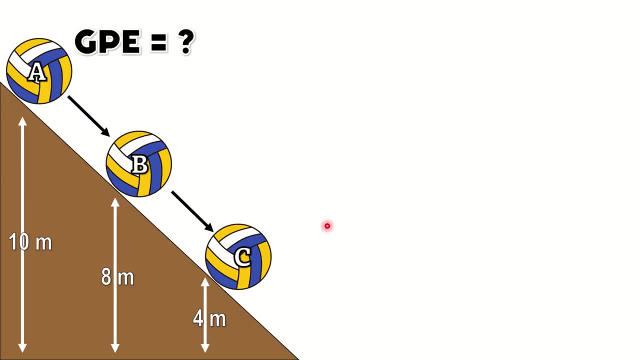 KE is equal to the one half of mass times the squared of velocity. Let's have a sample problem, As you can see in our illustration. let us determine the GPE, or the gravitational potential energy, of the ball at the point A, If the ball has a mass of 0.1 kilogram. 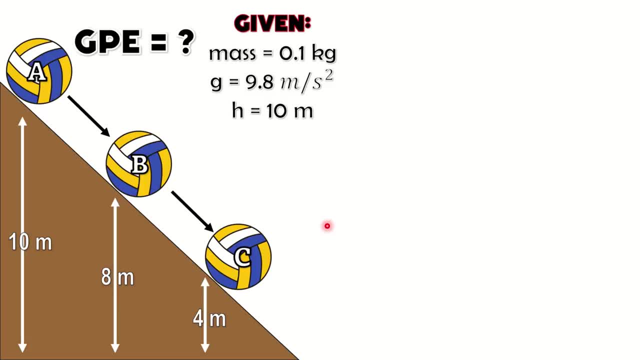 and the gravity of course is 9.8 meter per second squared and the height is 10 meters. let us find its GPE using this formula. Let us substitute the given to our formula and we have 0.1 times 9.8 times 10.. 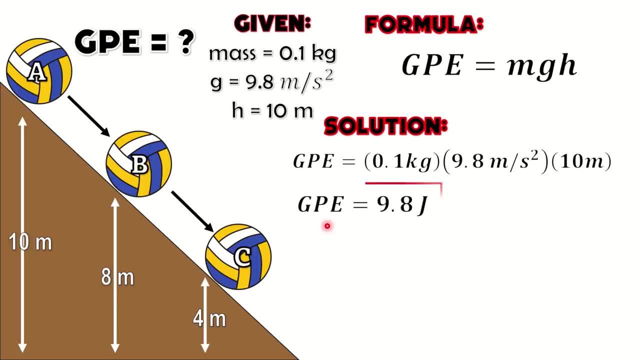 The product will be 9.8 joules. Remember, class, that the unit to represent energy is joules. Now we can also determine the value of the total energy. Since the ball is at rest, it has no kinetic energy, or KE is 0.. 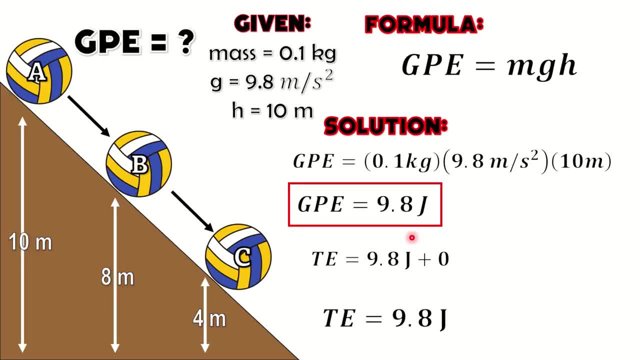 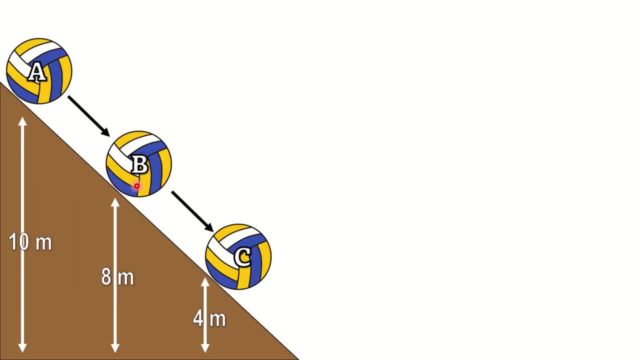 Thus the total mechanical energy of the ball is 9.8 joules. If the ball moves downhill, some gravitational energy gets transformed to kinetic energy. At point B there is a change in potential and kinetic energy. The gravitational potential energy decreases. 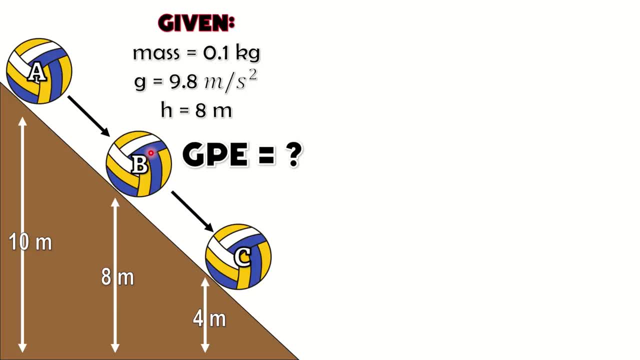 Let us calculate its GPE Again. these are our given and our formula. Let us substitute 0.1 times 9.8 times 8.. We have the product of 7.84 and our unit is joules. That is our final answer. 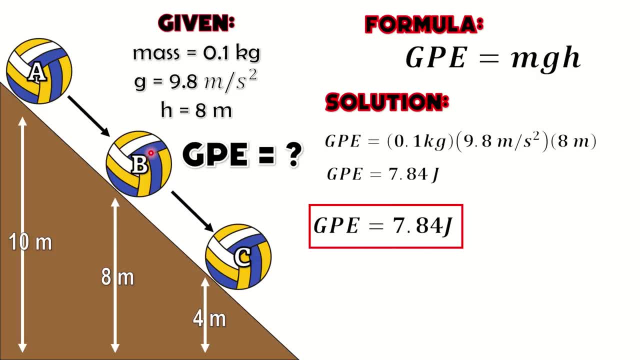 We can also calculate for the kinetic energy of the ball using the formula: TE is equal to PE plus KE. We all know that the value of total energy- the one that we got a while ago- is 9.8 joules and our gravitational potential energy is 7.84.. 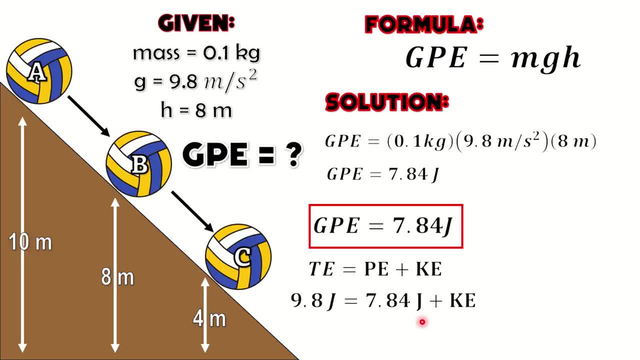 We can transpose this into the other side of the equation, and we know that transposing makes the sign opposite. Therefore, it will become 9.8 minus 7.84.. Our kinetic energy will be 1.96 joules. That is how you are going to solve it. 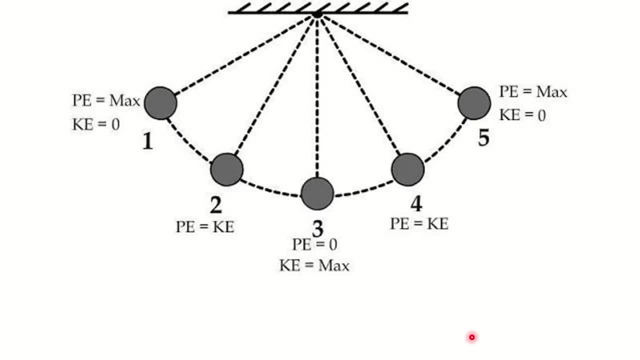 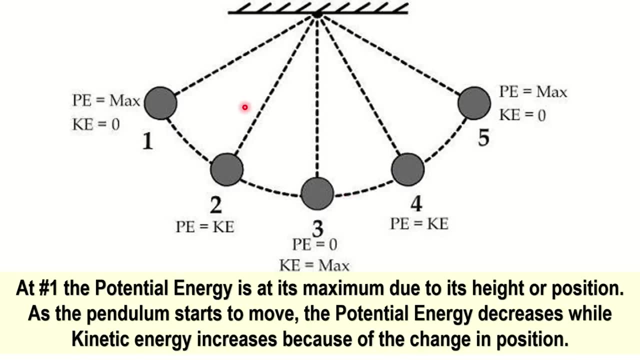 Class. Now let us have a swinging pendulum as another example. Let us analyze the mechanical energy in this pendulum. At number 1, the potential energy is at its maximum due to its height or position As the pendulum starts to move. 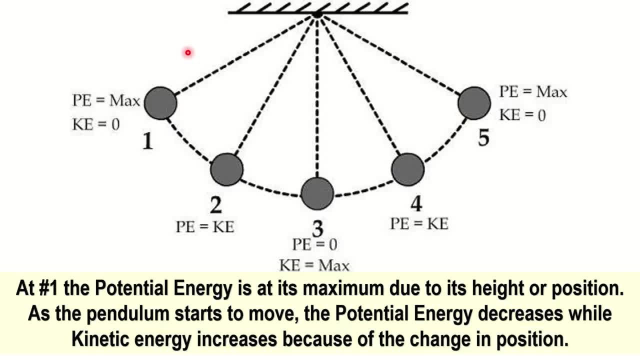 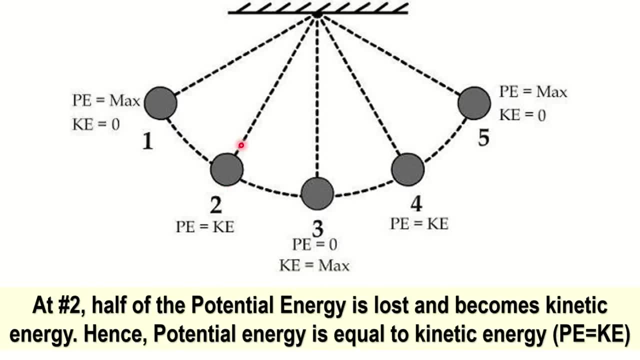 the potential energy decreases, while kinetic energy increases because of the change in position At number 2, half of the potential energy is lost and becomes kinetic energy. Hence potential energy is equal to kinetic energy, or PE is equal to KE. At number 3,. 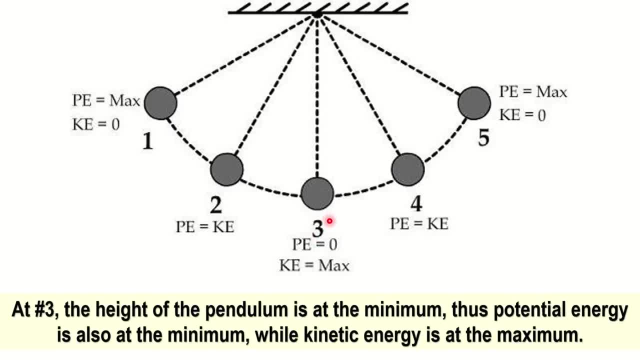 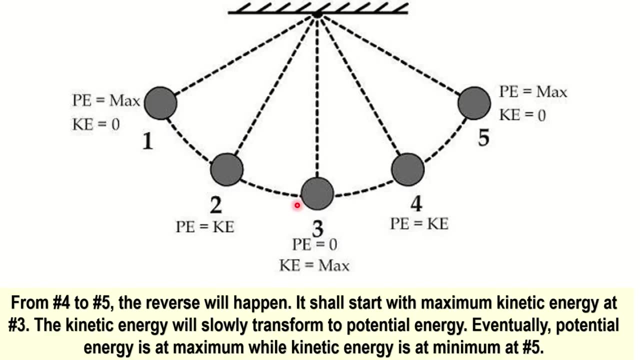 the height of the pendulum is at the minimum. Thus potential energy is also at the minimum, while kinetic energy is at the maximum. From number 4 to number 5, the reverse will happen. It shall start with maximum kinetic energy at number 3.. 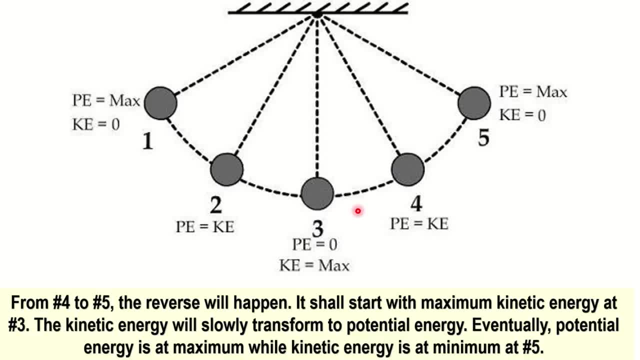 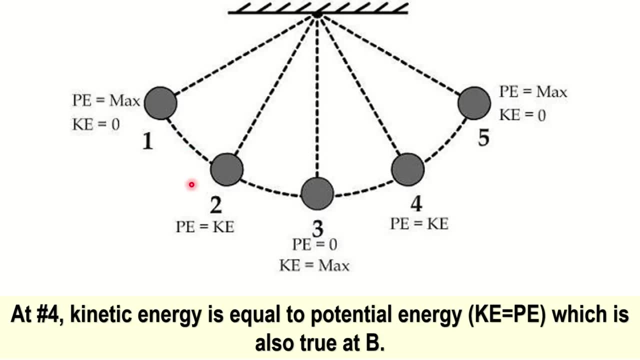 The kinetic energy will slow down and fully transform to potential energy. Eventually, potential energy is at maximum, while kinetic energy is at minimum at number 5.. At number 4, kinetic energy is equal to the potential energy, which is also true at number 2..